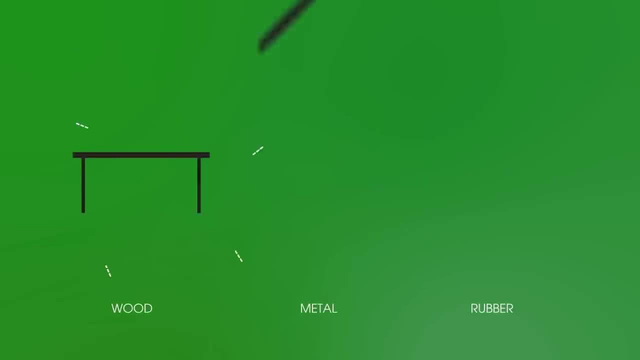 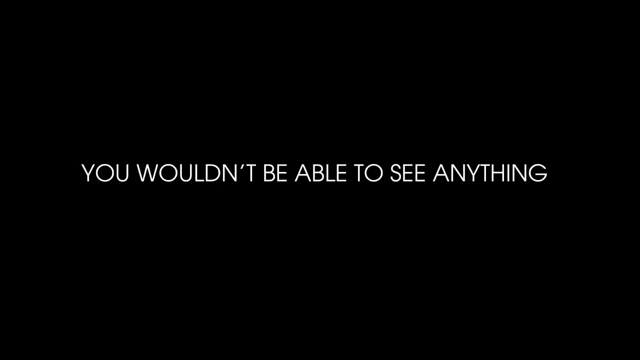 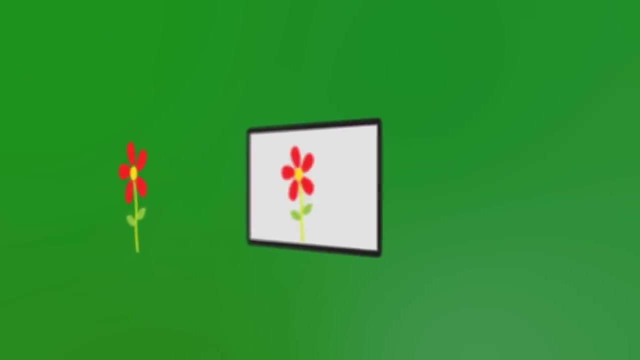 Reflection: Almost all surfaces reflect light. Otherwise we wouldn't be able to see anything. However, some surfaces are better at it than others. Shiny, silvery surfaces are best, and we use these in mirrors. So let's look at a simple plain mirror. By plain, we just mean 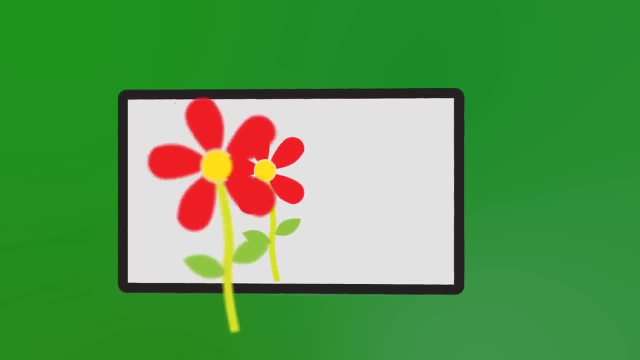 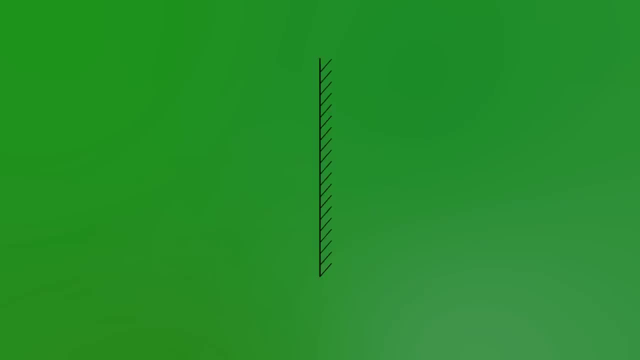 flat. Let's also look at how an image is formed in it. First off, we draw a mirror, And in physics we use a line with slashes on the back. so we know which is the shiny part. Let's look at a lovely, pretty flower. Now, every single bit of the flower is reflecting. 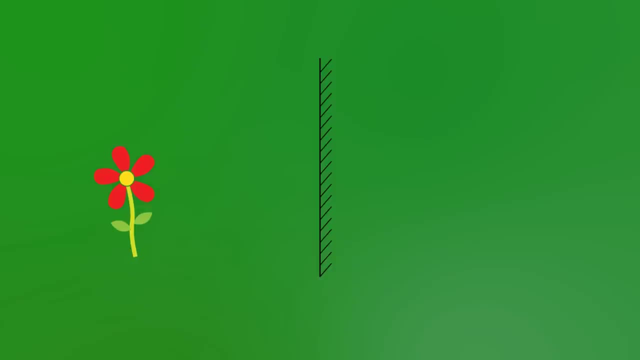 light, but we only need to look at one point. We'll choose a point at the top. Now, light is reflecting off this point in all directions, but we only really need to choose two, And it doesn't matter which two, as long as they hit the mirror. So let's draw those two. 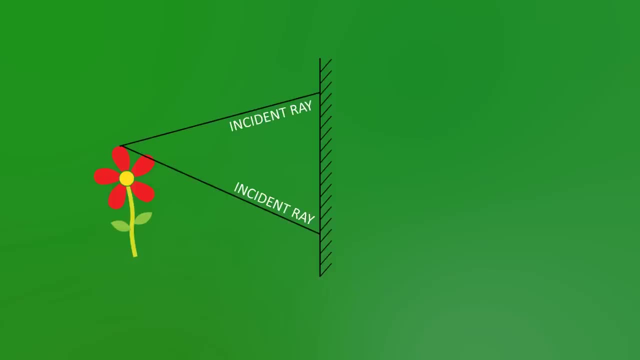 rays. Now, rays have to be drawn as straight, solid lines and they must have an arrow on to indicate their direction. Both these rays are called incident rays, as they're incident on the mirror. Okay, now for our first rule. Whenever a light ray hits a surface, we must draw a normal 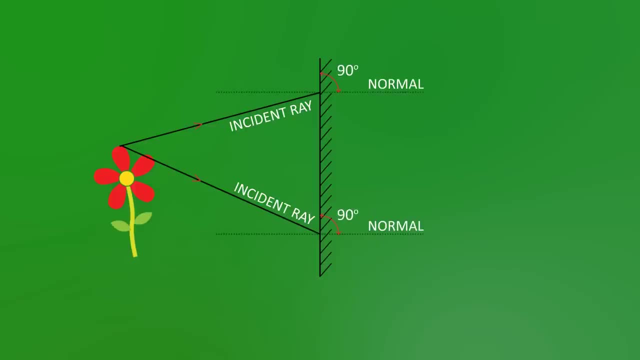 This is a dotted line at 90 degrees to the surface, where the light ray hits, And we always measure angles. We measure angles between the normal and the ray. This is because we sometimes have funny shapes. Right now, we've drawn our normals, we can add our reflected ray. Now, our reflected rays. 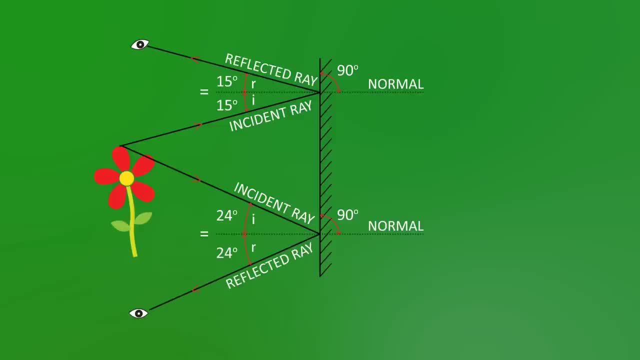 will bounce off at the same angle that the incident rays hit, just like a bouncy ball would off a table. This is the law of reflection Angle. I must equal angle R. Now we've got the two reflected rays. The second rule. 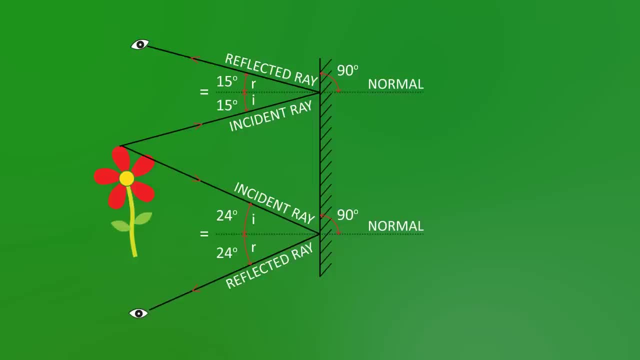 The second rule. These are what will actually be seen, But we always focus rays as if they've come from a single point, But these two haven't, So where will we think they've come from? Let's trace them back using a dotted line and see where they cross.